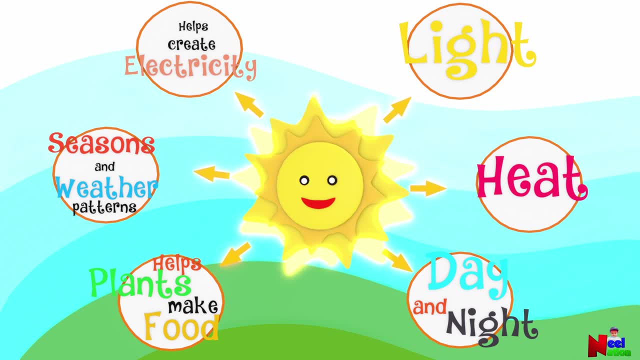 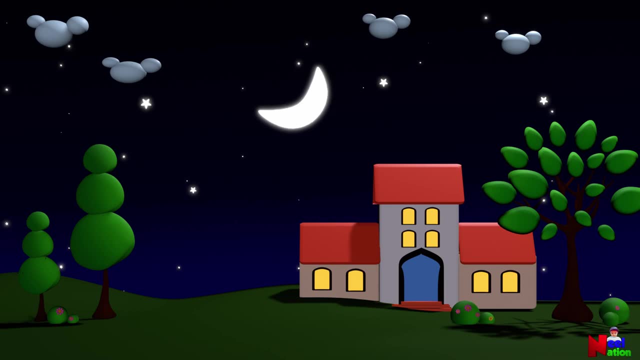 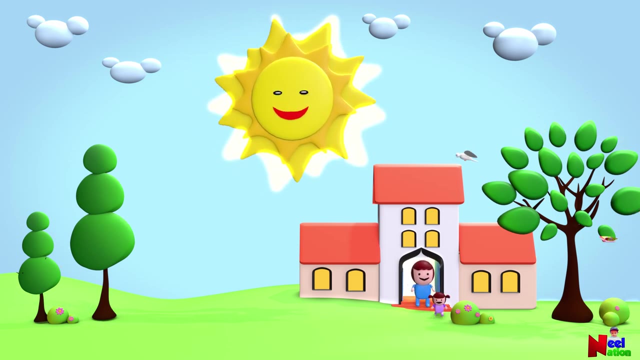 Light, Heat, Day and night, Food, Seasons and electricity. One of the most important things the sun does for earth is to provide us with the light. When the sun shines on earth, it lights up everything around us so we can see. 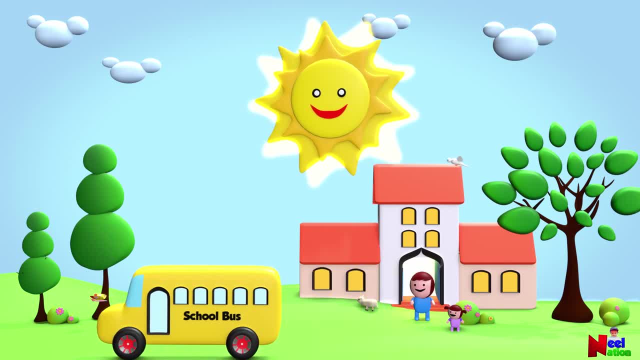 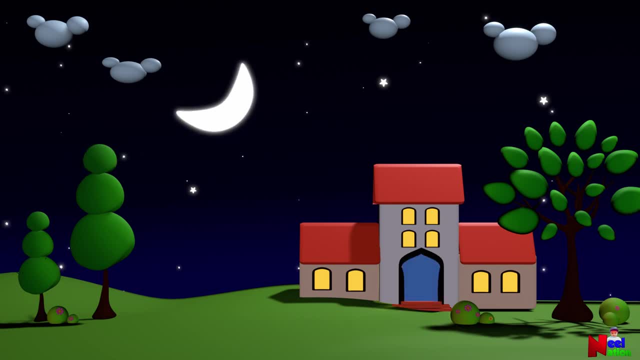 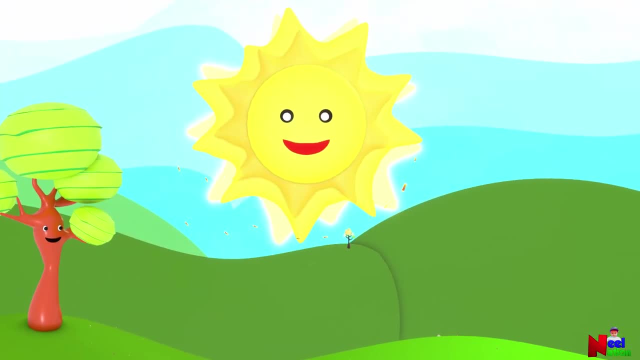 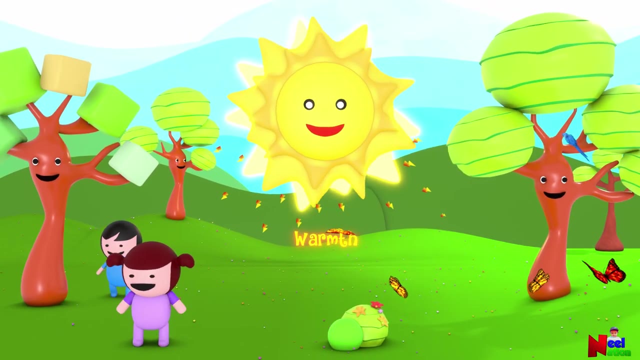 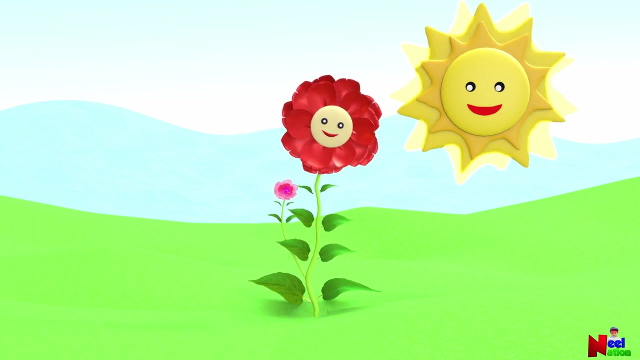 Sun gives us light. Sun also provides us with warmth. When the sun's rays reach earth, they heat up the air and the ground. This warmth is what makes earth a comfortable place to live. Sun gives us heat. Energy is like fuel for our bodies, and we get it by eating food or, in the case of plants, through. 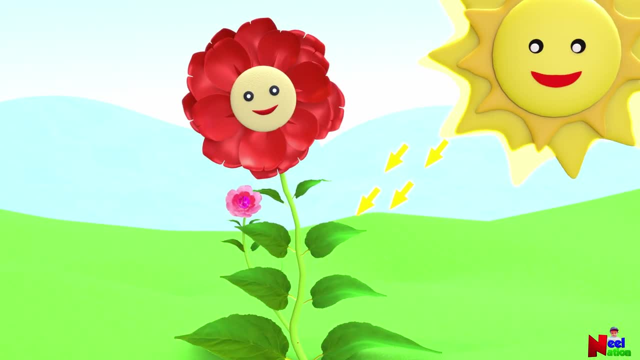 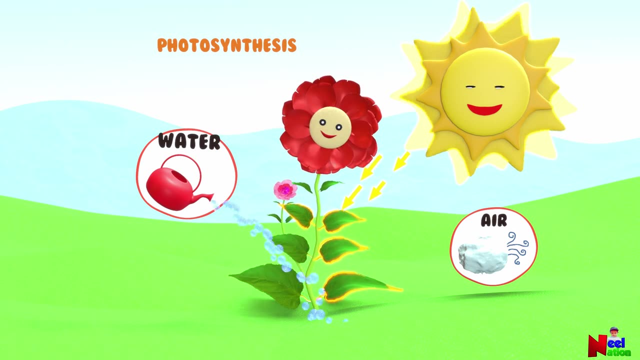 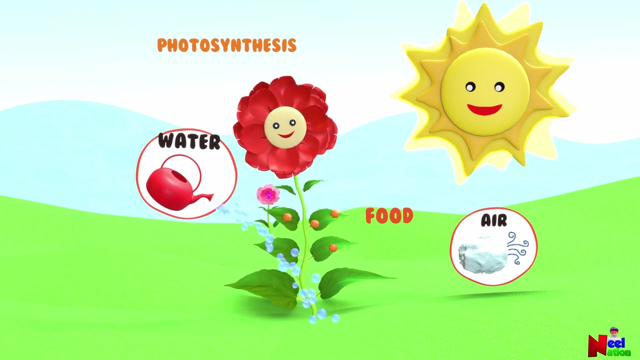 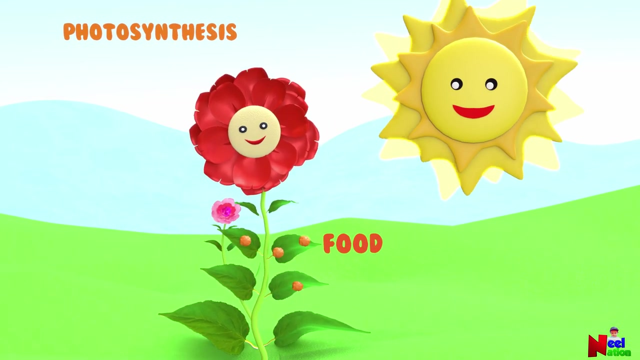 photosynthesis. Green plants make their own food. through a process called photosynthesis, Plants, with the help of energy from the sunlight, water and air, make their own food. Food is used by plants to grow, form flowers and develop fruits. Sun helps plants make food. 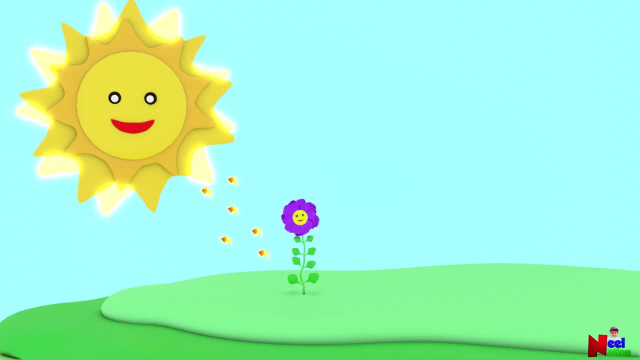 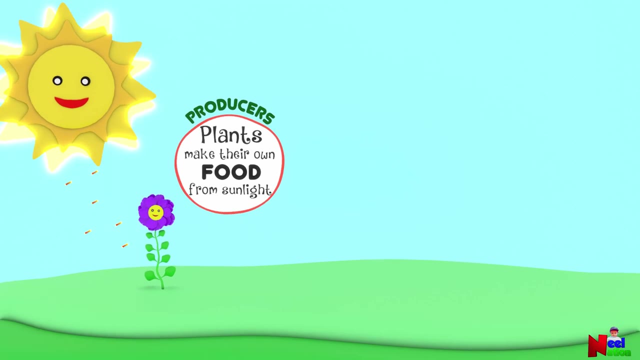 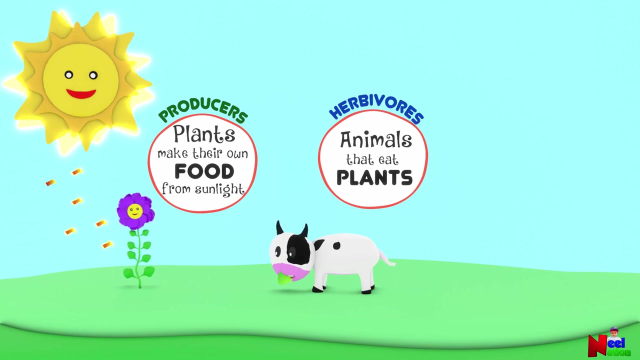 Plants are also called producers, as they can make their own food with the help of sunlight Producers. Producers, Producers- There are some animals called herbivores. They get energy from eating plants. Herbivores- Cows, deers and rabbits are some of the herbivores. 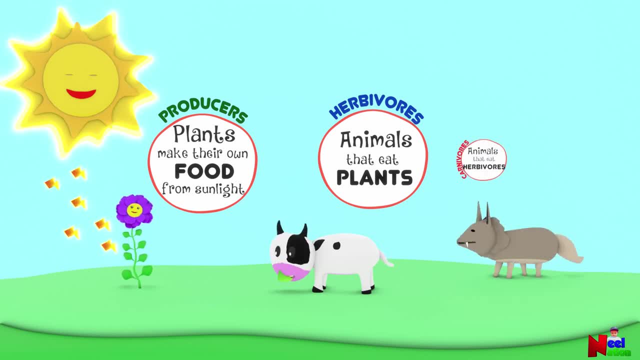 Some animals, called carnivores, eat other animals to get energy. Wolves, lions and snakes are some of the carnivores. Carnivores, In other words. though, indirectly, the sun provides food to all animals through plants. This transfer of energy from plants to animals and to other animals 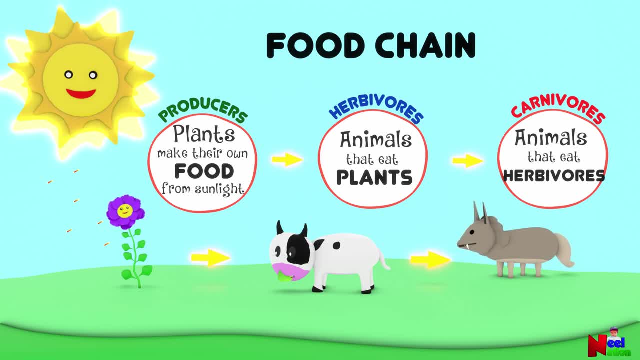 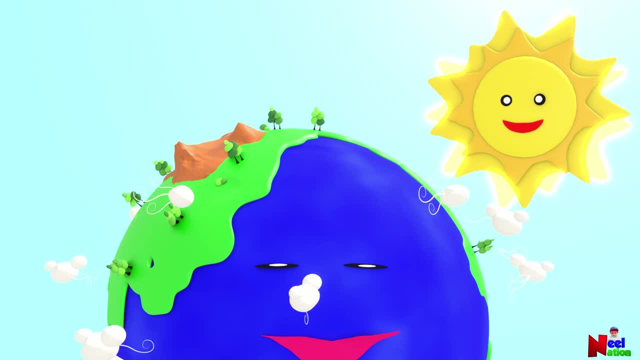 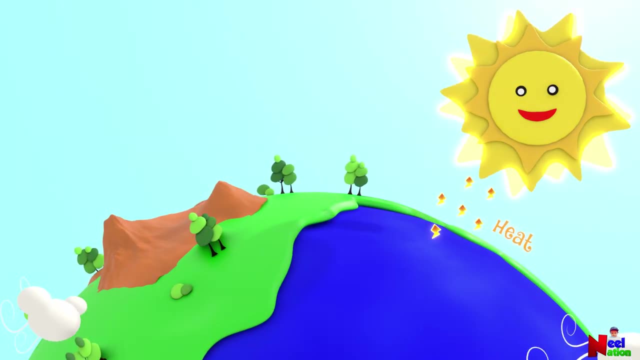 is called the food chain. The sun helps create weather patterns on earth. The sun's energy causes air to move around, which can create wind and rain. The sun heats the surface water of lakes and oceans. When the water gets hot enough, it turns into a gas called water vapor, which rises up into 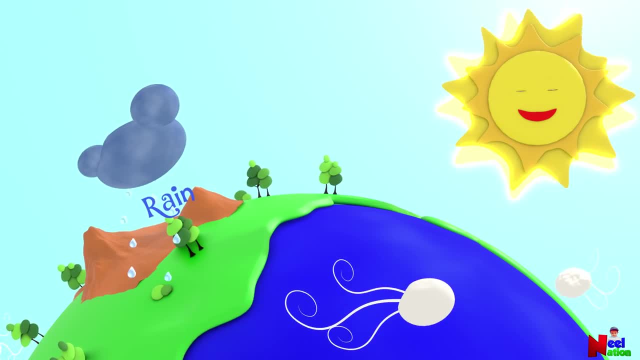 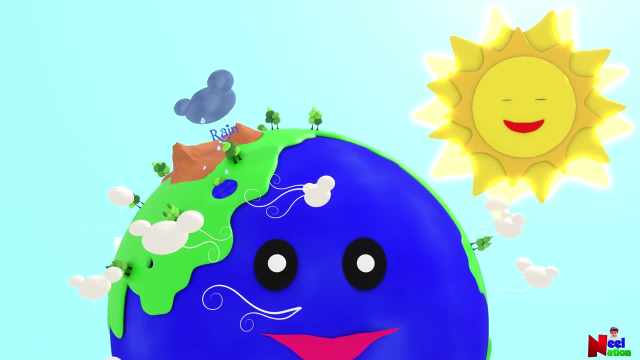 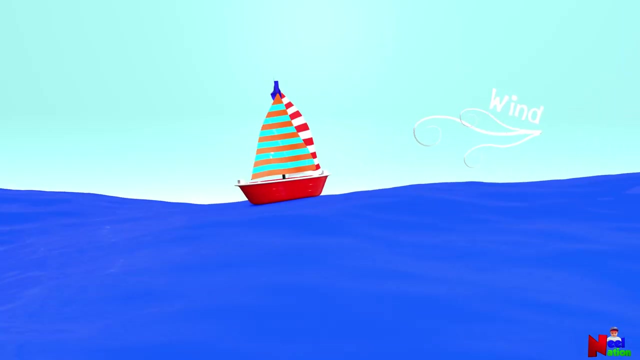 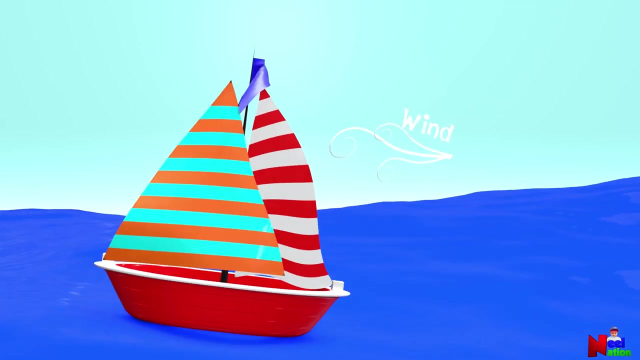 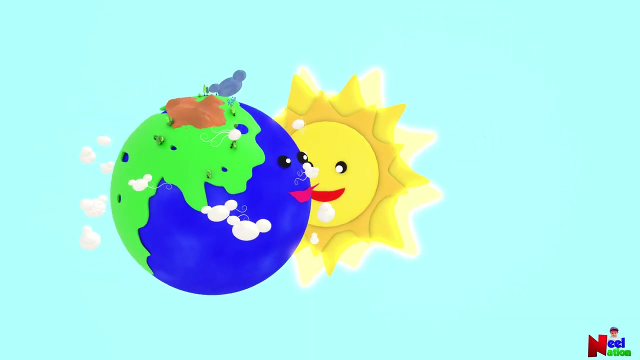 the sky. Then it forms clouds, falls as rain and collects in lakes and rivers. Sun uses rain and wind. Wind energy can be used to power boats and other vehicles. Wind energy can also be used to make electricity. Wow, The sun also gives us seasons. As the earth orbits around the sun. the angle of the sunlight. 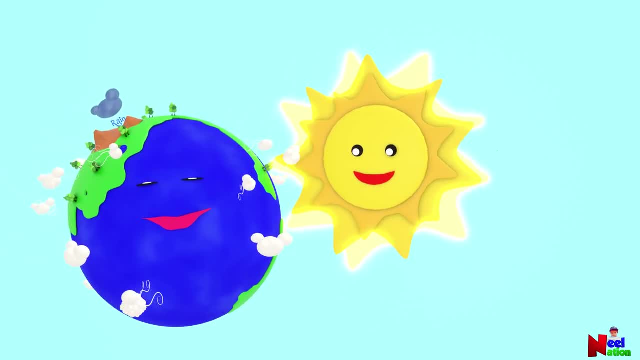 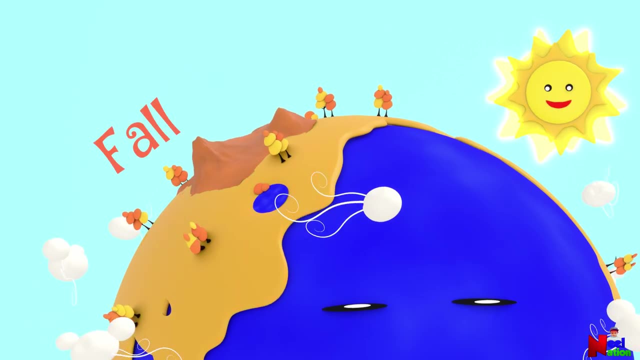 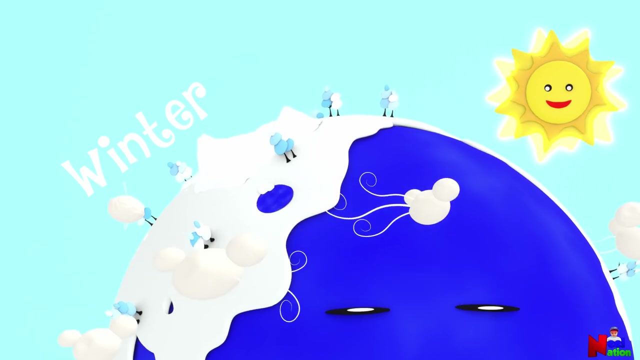 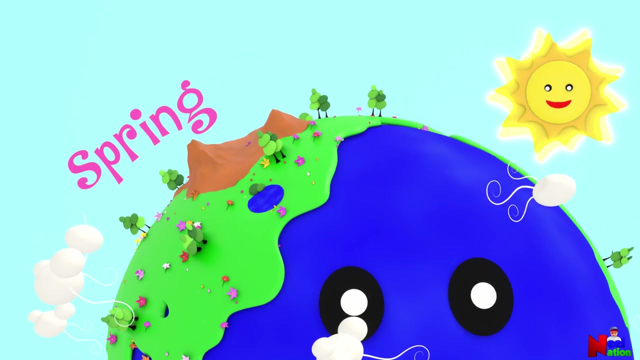 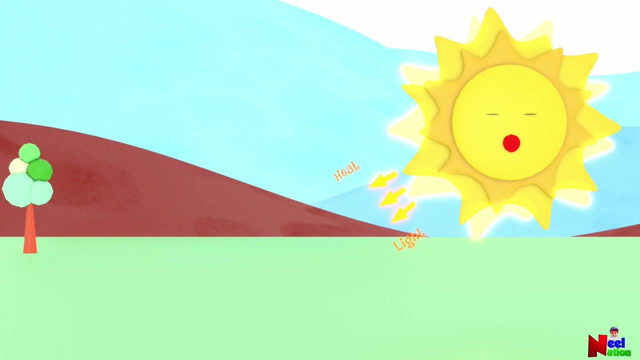 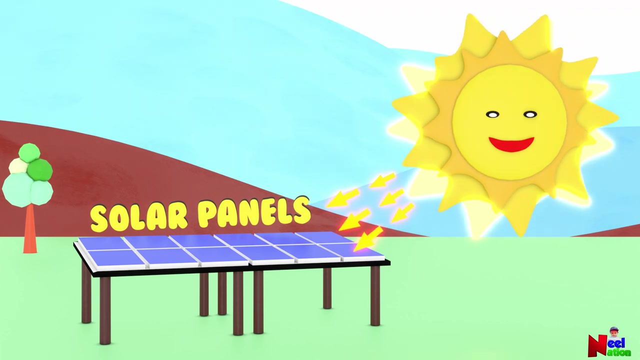 changes, which creates different seasons like summer, fall, winter and spring And spring. Sun uses weather and seasons. The heat and light from the sun can be used to create electricity. This is done using special devices called solar panels. Solar panels are made up of smaller units called solar cells. 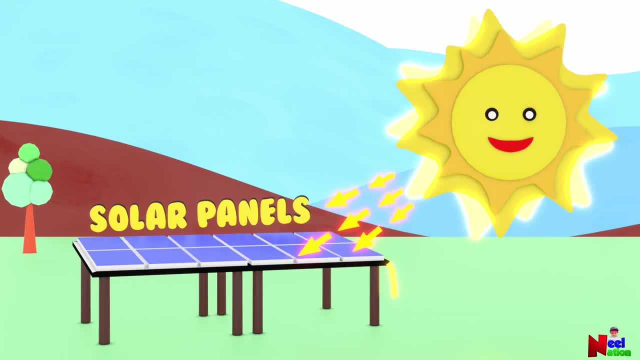 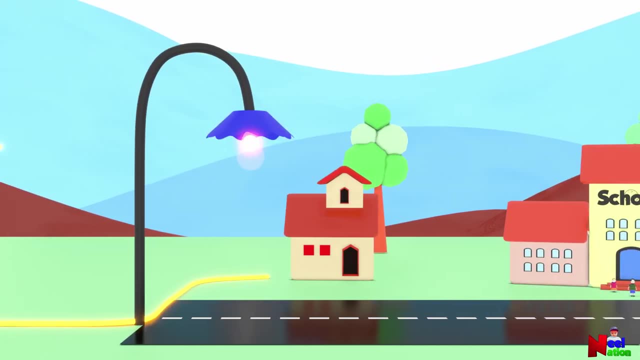 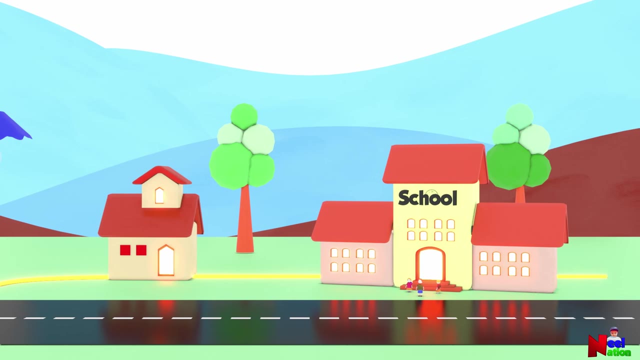 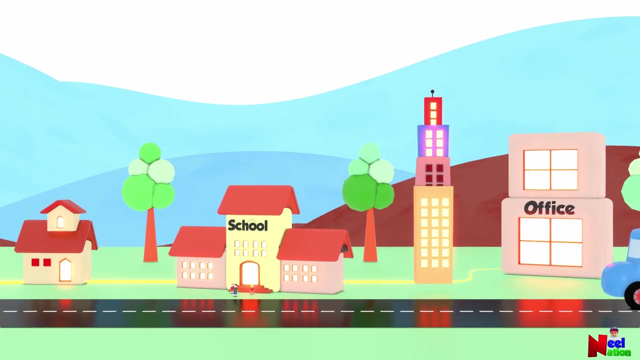 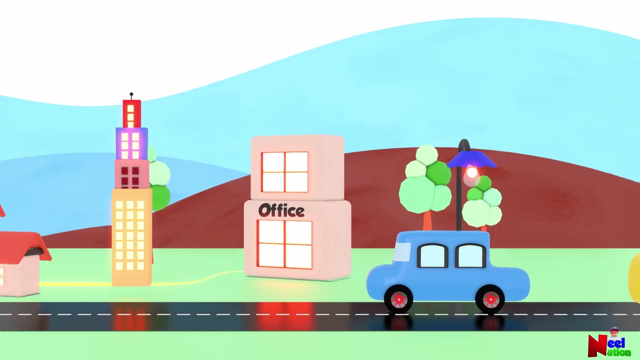 When the sun's light hits these cells, it creates electricity. This electricity can then be used to power things like homes, schools and businesses. Electricity can also be used to power electric cars, trains and buses. Sun uses electricity. It's a power station. 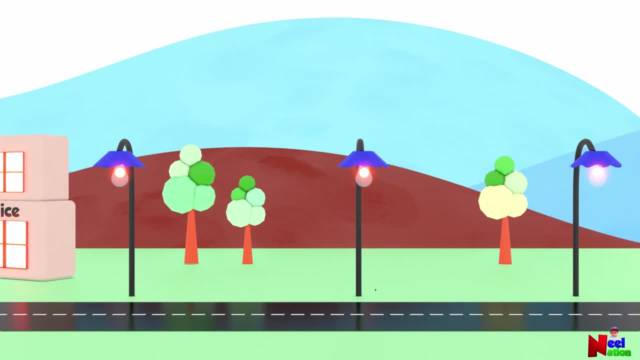 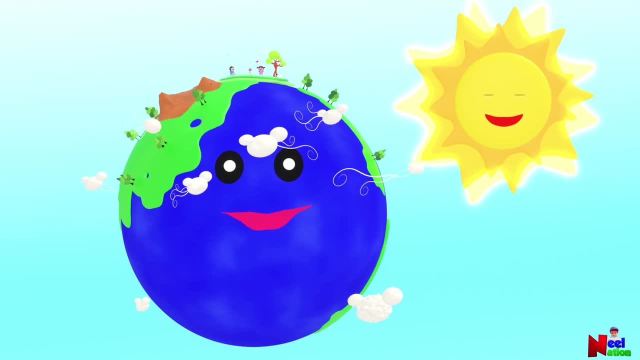 It's a power station. It's a power station, It's awesome. Solar power is a really great way to make electricity because it's renewable, Which means it won't run out. like other sources of energy, It can be used over and over again. 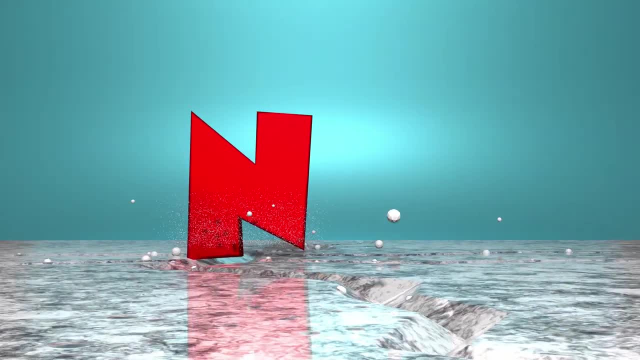 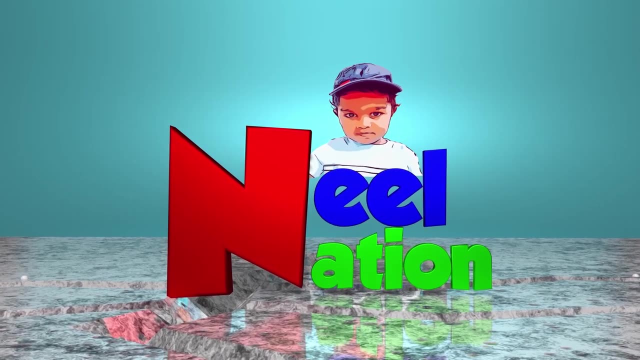 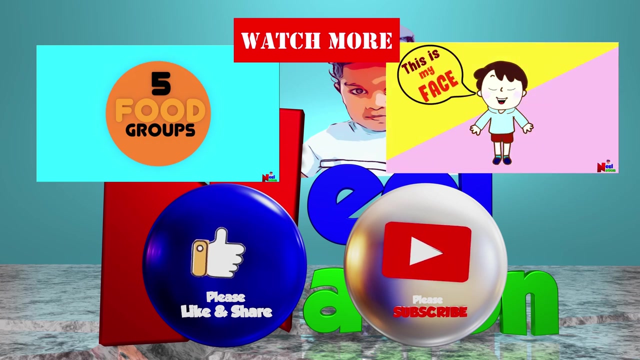 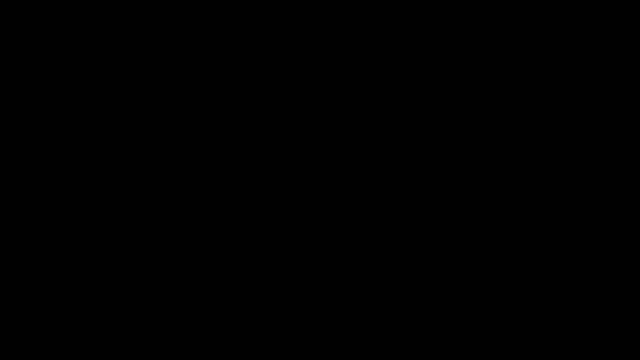